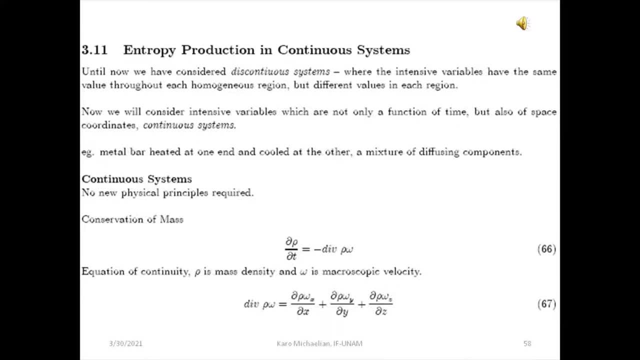 So this equation 66 is the continuity equation, or the variation of the mass density in time, which is just equal to minus the divergence of the mass density times the velocity of the flow of the matter coming into or out of the system. So this equation 66 might look a little bit mysterious, but in fact it comes from Gauss's law, in which the change or the rate of change of a variable of the system 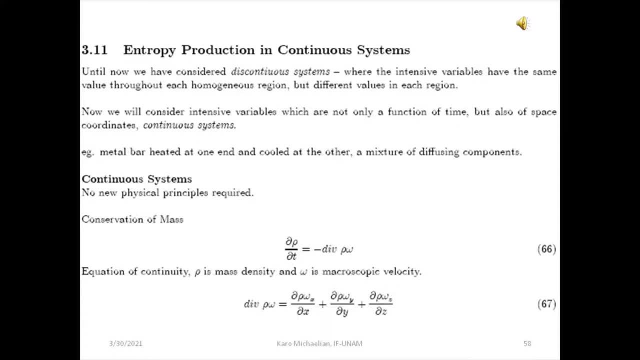 the system, within a well-defined volume to the given surface, is just equal to the flow, the normal component of the flow integrated over that surface. Or, using Gauss's law, it is just equal to minus the divergence of the flow over the volume that that surface is bounding. 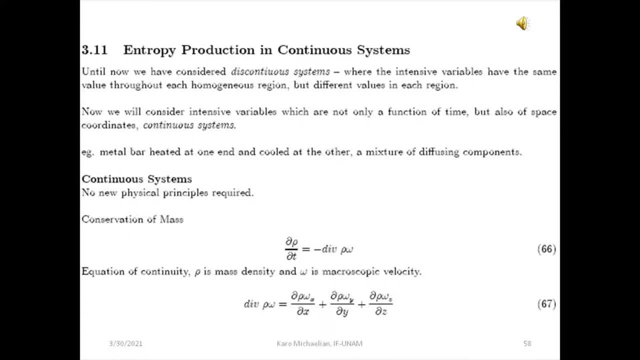 So this equation 66 is just the equation of continuity, or the mass density, rho, and where omega, the vector, is the macroscopic velocity of the material which is moving in the system. And I will remind you that divergence is just given by this mathematical formula, which is 67,. equation 67. 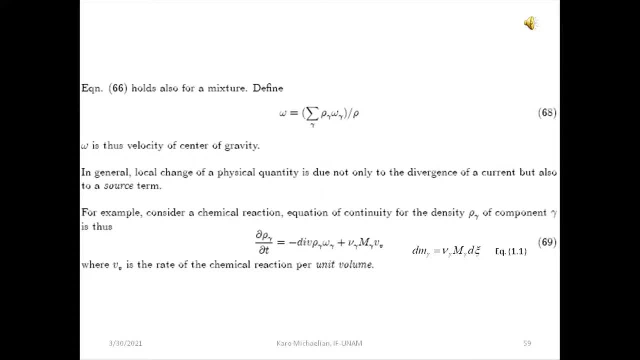 Now equation 66,. the continuity equation also holds for a mixture of different components, So in this case, omega then refers to the velocity of the center of gravity, which is just defined, as omega is equal to the sum over all the components in the system. 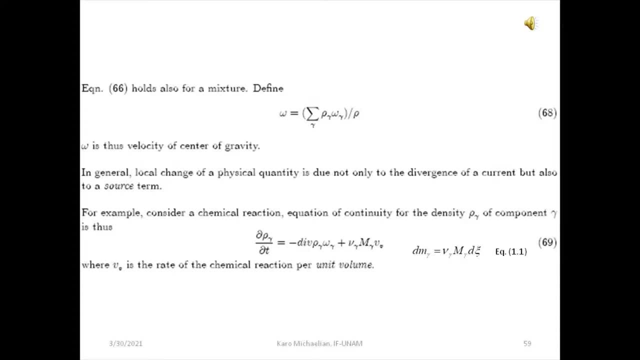 of the densities. the mass densities of those components times the velocity of the flow of those components over the total density, rho. In general, the local change of a physical quantity is due not only to the divergence of a current but also to a source term. 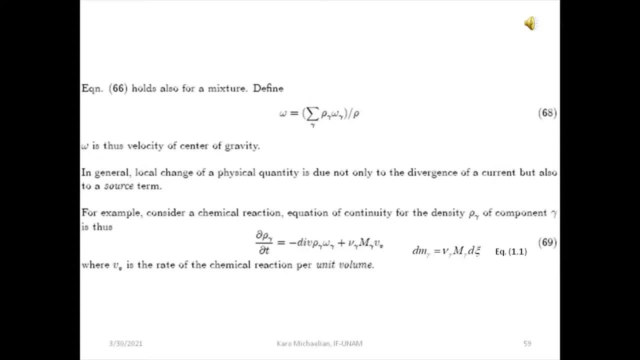 For example, if we consider a chemical reaction in which we are producing certain components, gamma, the equation of continuity for the mass density rho gamma, that is, the mass density of component gamma, is just this equation 69, in which we have included the second term. 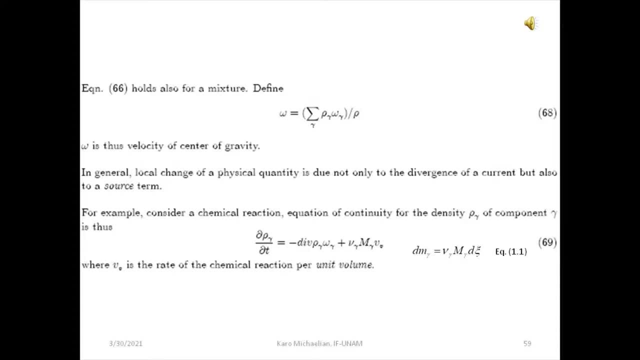 which are due to the production of that component gamma, Due to the chemical reactions. And we can see that if we go back to equation 1.1, from the book of Prigogine, where dm gamma is just equal to the stoichiometric coefficient gamma times the molar mass of substance gamma. 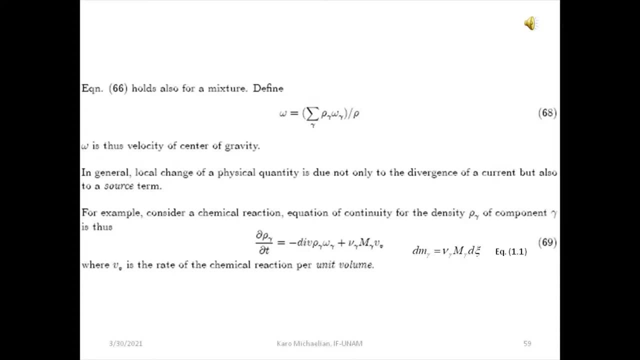 times d chi, which is, remember, chi is the advancement of the reaction, So d chi by dt is the velocity of the reaction, Or in other words, the rate of the chemical reaction. The rate of the chemical reaction per unit volume. 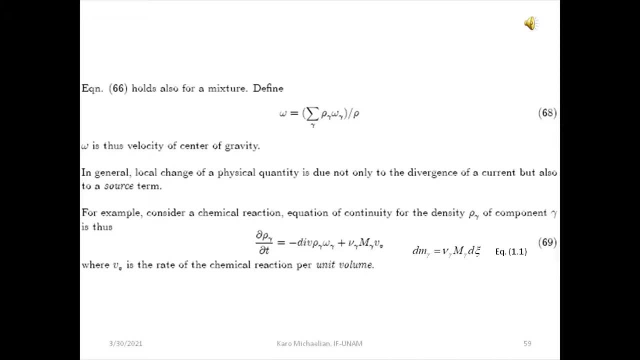 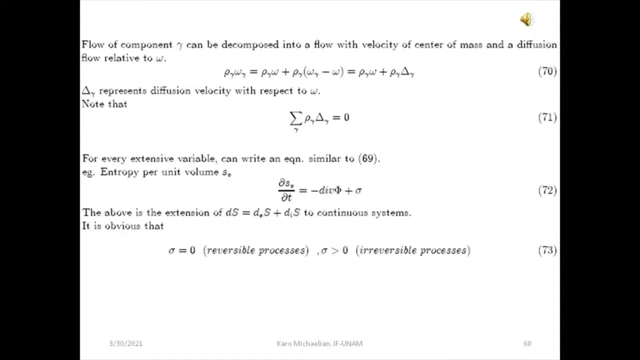 Now we have to talk about all substances per unit volume, Because now we are considering a continuous, not a discrete case. For any component gamma in the system, the flow can be decomposed into a flow with respect to the center of mass of the system. 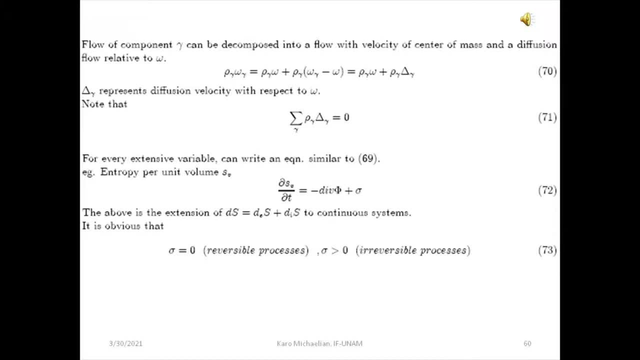 and the diffusion with respect to the flow, relative to the center of mass velocity. So, for example, we can write rho gamma, omega. gamma, which is equal to rho gamma times, omega. omega, remember, is the center of mass velocity of the system. 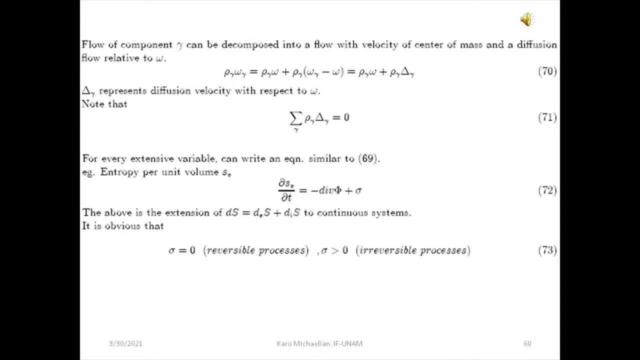 plus rho gamma times the difference of the velocity of the component gamma with respect to the velocity of the center of mass of the system. So here in this equation 70, delta refers to the diffusion velocity with respect to the center of mass of the velocity of the system. 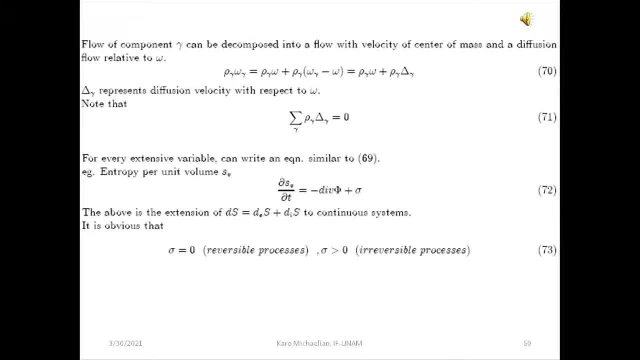 And note that by our definition- equation 70, of the diffusion velocity with respect to the center of mass velocity, we know that the sum over all components of their densities times their diffusion velocity with respect to the center of mass of the system has to be equal to zero. 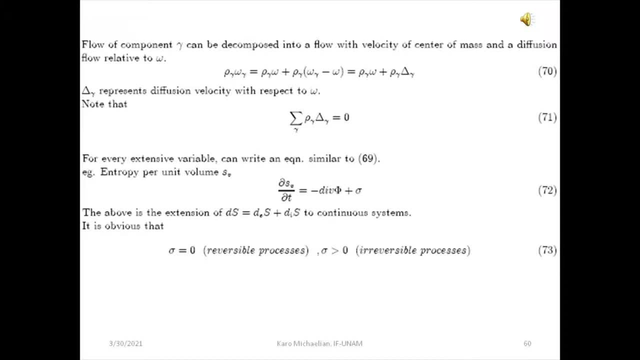 So not only for the mass density but for every extensive variable, we can write an equation very similar to equation 69. For example, for the entropy for unit volume we have a term which is equal to the divergence plus another term. 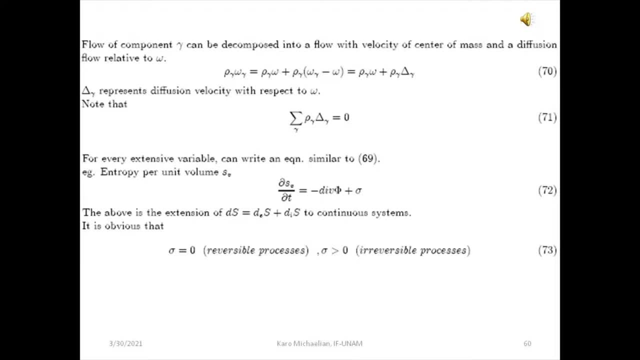 sigma, which is equal to the production. The divergence is the flow of entropy over the boundary of the system and sigma is the production due to irreversible processes occurring inside the system. So equation 72 is just an extension of the change of entropy being equal to. 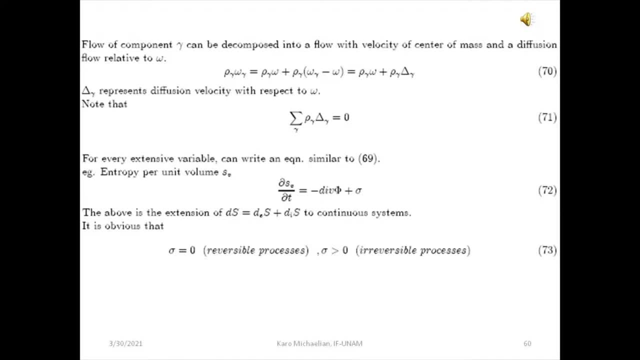 the change of entropy due to the flows of entropy coming in from the outside of the external environment or going out of the external environment, plus another term which is due to the internal entropy production of the system. So this equation ds is equal to. 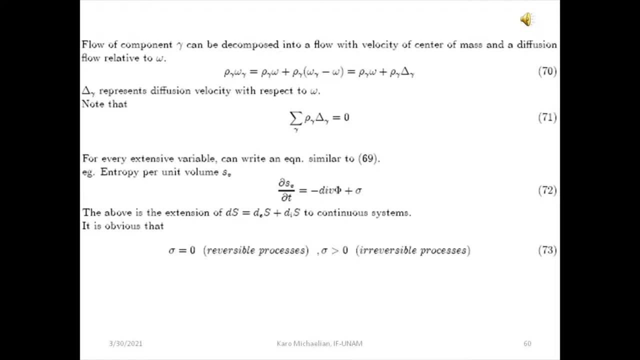 dEs plus dIs is just exactly equation 72, but for the case of a discrete system, which we treated before, Now we're going to treat continuous systems, so we will have to use equation 72,, which includes a divergence of the flow. 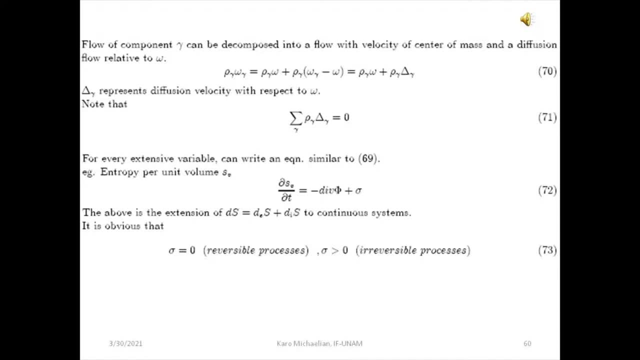 the entropy, in this case plus another term, sigma, which is equal to the entropy production due to irreversible processes. And note that for reversible processes, the production of entropy is equal to zero, sigma is equal to zero, while for all irreversible processes occurring within the system. 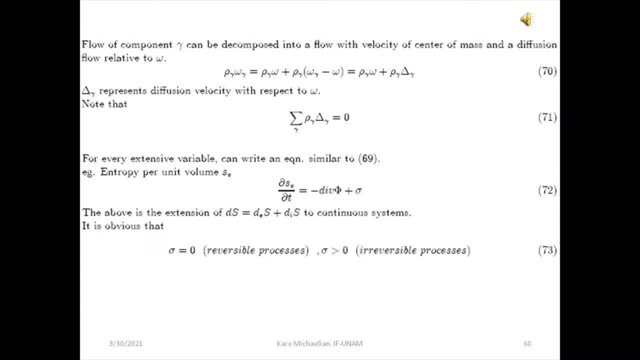 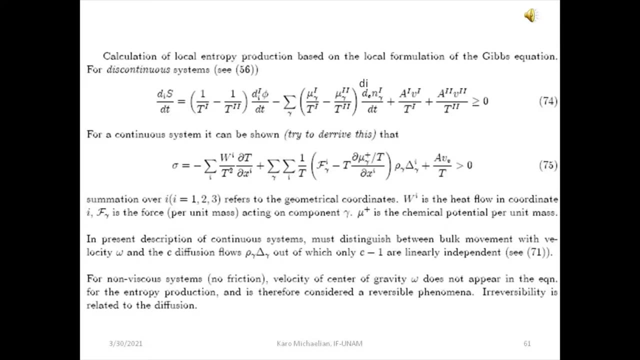 the entropy production has to be positive. definite sigma is greater than zero. equation 73.. So now let's calculate again the entropy production due to a system composed of two parts, one and two. okay, so this is the discrete case in which parts one and two. 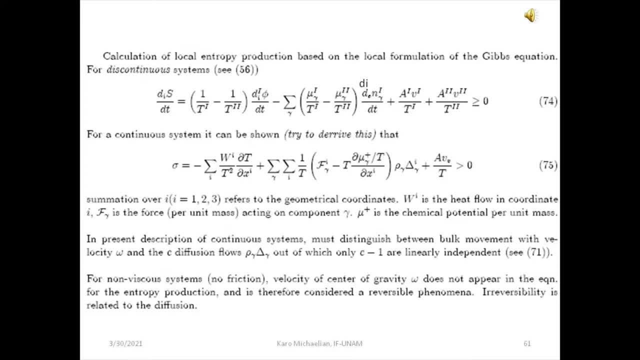 or regions one and two are open to each other, so we allow a flow of energy and matter from subsystem one into subsystem two and vice versa, and the system one plus two is closed as a whole. so we only allow a flow of energy. 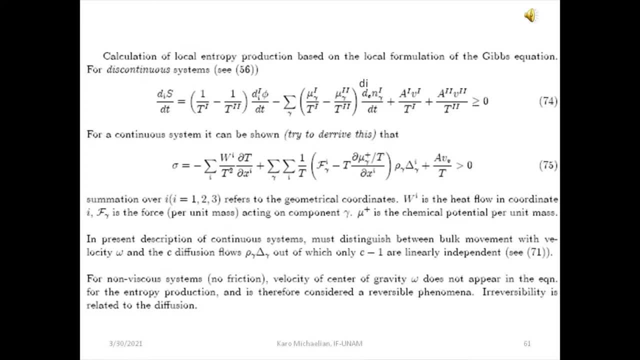 over the boundary of the system, the complete system, one plus two. but we don't allow a flow of matter over the whole system. So now, if you remember, this is the form that we derived for the entropy production for this system, and you can go back to equation 56 to see that. 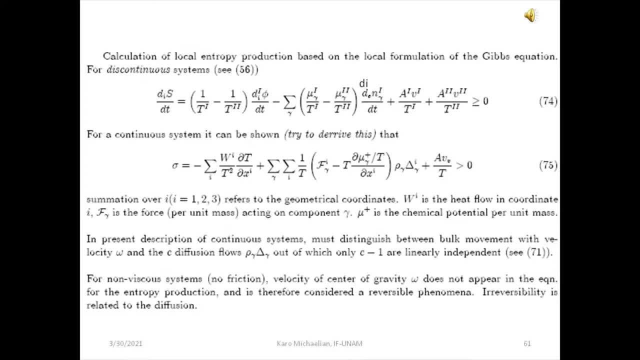 So the entropy production, internal entropy production, is just due to one term, which is the force- one over T1 minus one over T2, times the flow. in this case was the flow of heat plus the flow of energy. 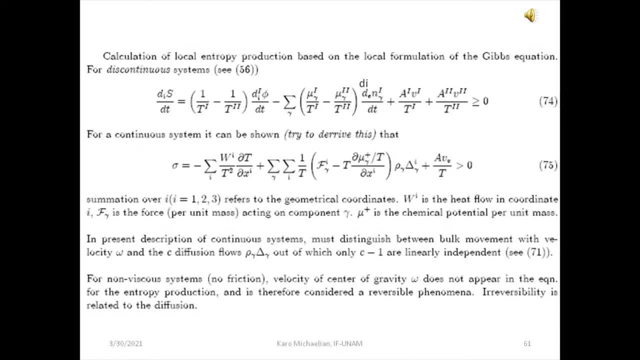 which is coming in from the matter, because we're allowing matter to flow between subsystem one and subsystem two. So the first term here was production of entropy due to the flow of energy. The second term is the production of entropy due to the flow of mass. 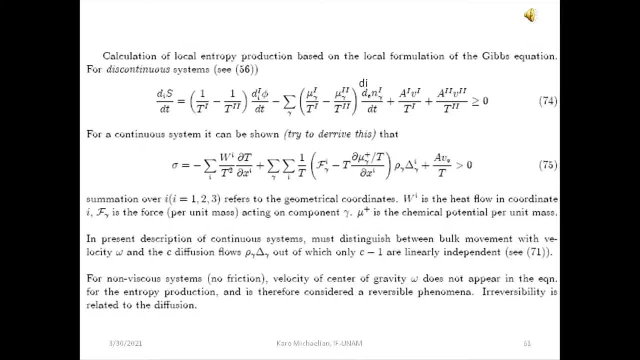 where the mu gammas are just the chemical potentials of the component gamma In system one and system two, over their temperatures, times the flow of the material of that substance, gamma. And the last two terms are due to the chemical reactions which are occurring. 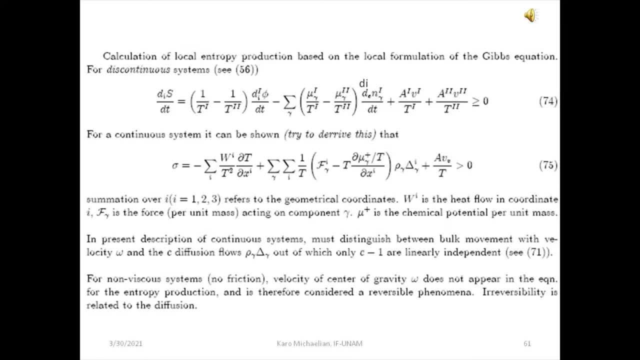 inside system one and system two. So they're the force for the chemical reactions, which is the affinity over the temperature, A, over T- and the flow is the velocity or the rate of the reaction. V rate of the chemical reaction. 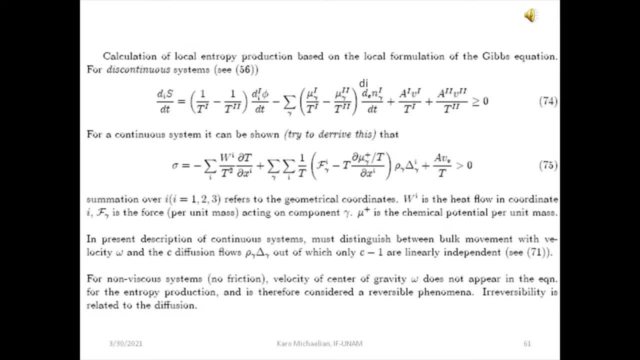 So now, rather than a discrete system, we assume that we have a continuous system. We ask how equation 74 would look, the case of a continuous system. We won't derive it here, but you can try to derive it for yourself. Equation 75. 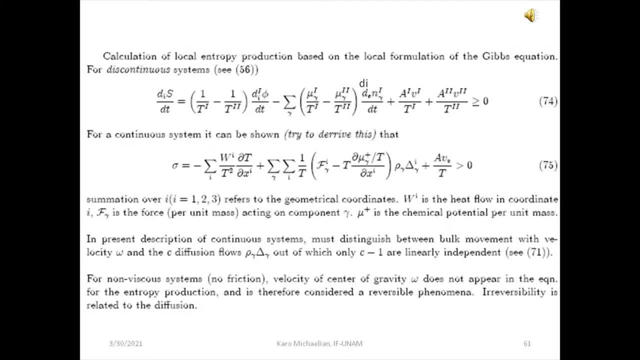 is the corresponding continuous case for equation 74 for this system that we have, of a system being open to flow of material and energy inside that flows on its boundary and only allowing a flow of energy over the boundary. So the first term here is W. 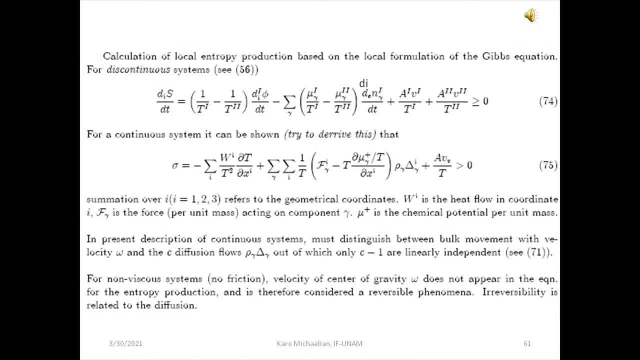 I with the, with the superindex, I represents the flow of heat in the coordinate I. So this I is the sum over three coordinates- X, Y and Z- of the system, And it is multiplied by a term, partial, T. 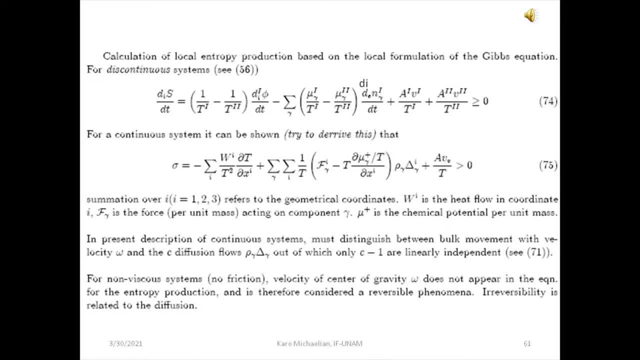 the temperature with respect to X, the X coordinate. No, it can be X, Y or Z. That's why subindex I appears there over the temperature squared. That first term corresponds to the first term in equation 74. 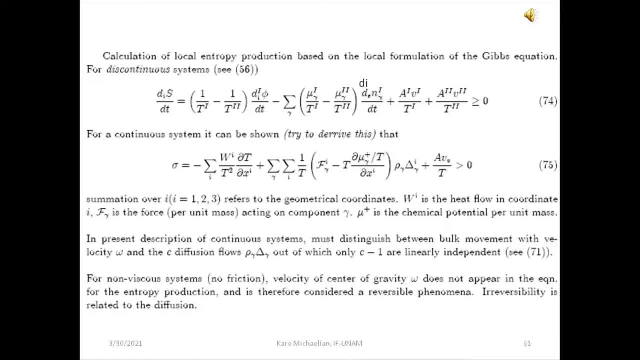 for the flow of heat, flow of energy in the system. Now, the entropy production due to the flow of matter in the system, in this continuous system, is just this second component of the equation 75,, second term, which is the sum overall. 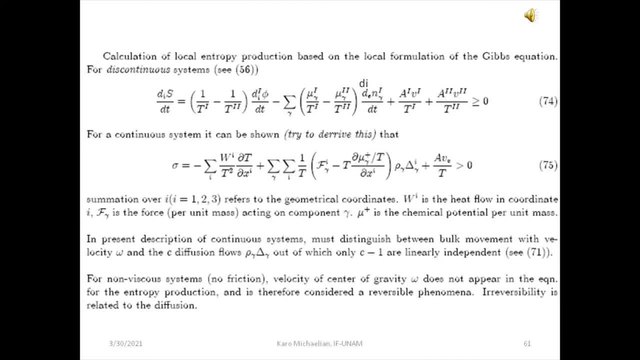 of the components gamma in the system which are diffusing. this is the diffusing, this is the diffusion term times a sum over all of the indices X, Y, Z, coordinate space And F. here this F is the force. 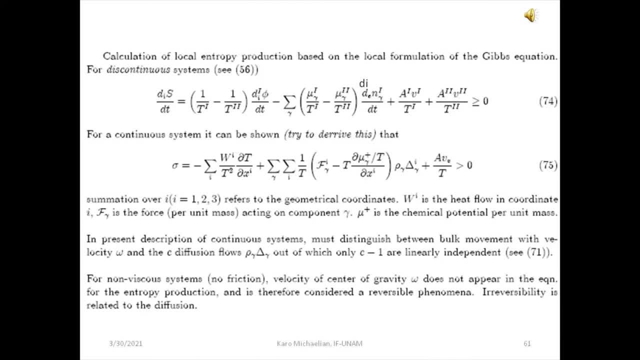 the external force. we're allowing, in this case, an external force to exist over the system, For example an electrical potential, which would provide a force if the components were charged in the system, And this minus T is called mu, Now here mu plus. 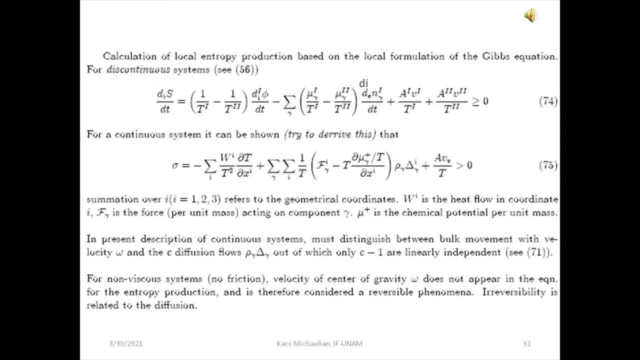 with this super-indice. E plus is the chemical potential per unit mass, because now we are looking at the volume, regional volume, so we have to do it per unit mass. over the temperature with respect to partial X, Y and Z. 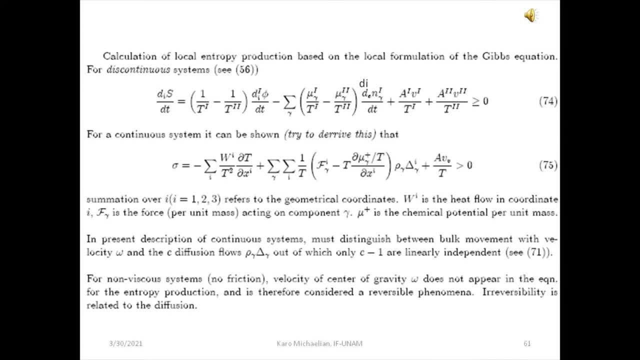 And it's multiplied by the mass density times. now, this delta, remember, is the velocity of component gamma with respect to the velocity of the center of mass of the system And in each of its three components, X, Y and Z. 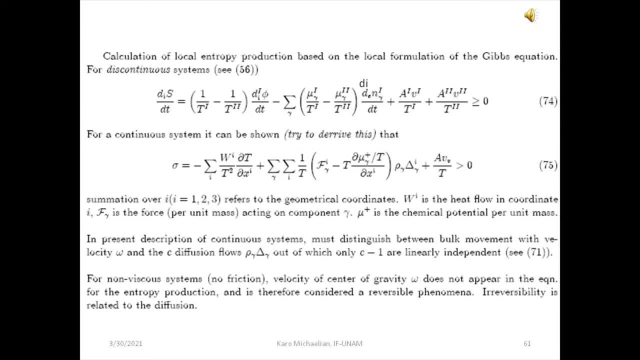 that's why the sum in the CI again, And then we just have a single term for the chemical reactions occurring in the system, which is the affinity over the temperature times, the rate of the reaction, V, And now by the local format. 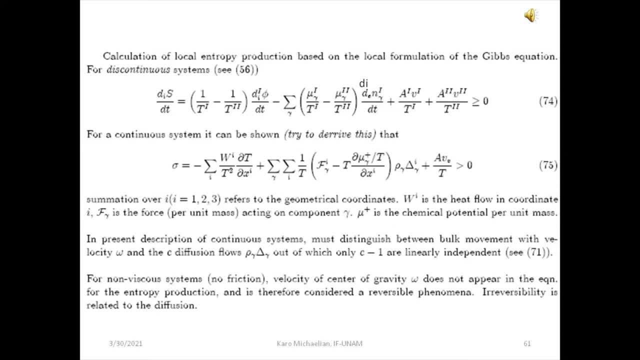 and the formulation of the second law of thermodynamics. this entropy production has to be positive definite. So here we're not going to derive equation 75. It should be fairly obvious that it is the correspondence of equation 74,. but for the continuous case, 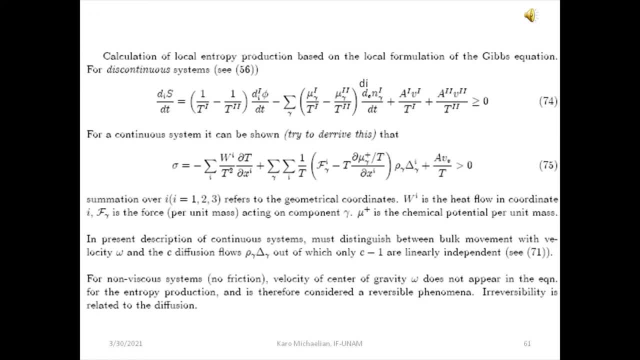 instead of the discrete case. Now, in the present description of continuous systems, we must distinguish between the bulk movement, the velocity omega- omega is the velocity of the center of mass of the system- and the C- this is the number C. 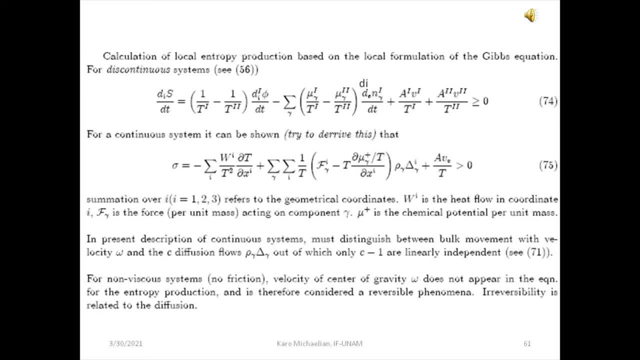 which is the number of different components in the system, the fusions of these different components with respect to that of the center of mass. So there are only really C minus 1 linearly independent variables. delta gamma: Now also note that we're not 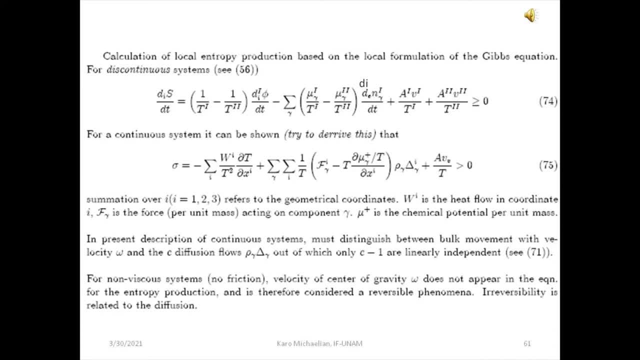 going to be able to determine what is the velocity of the center of mass of the system. We're going to be able to determine what is the velocity of the center of mass of the system Now. also note that we are considering non-viscous systems. 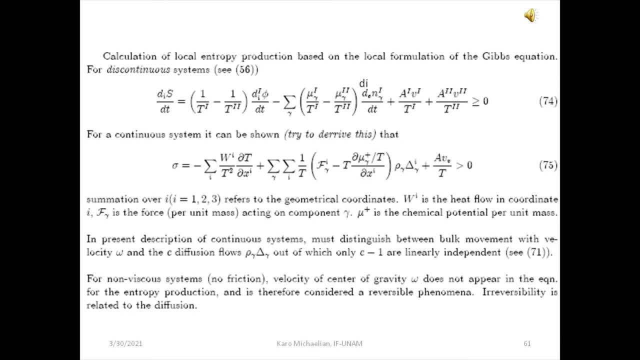 that is no friction with respect to the outside. So the flow of the center of mass does not appear in the equation for the entropy production. The entropy production is only due to the flows with respect of the, the flows of the different components with respect. 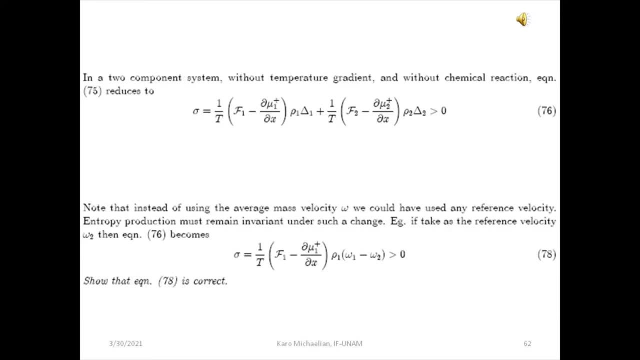 to the velocity of the center of mass of the system. So now let's consider a simple example of a continuous system. And this is an example of a continuous system. In this example we only allow two components. We have only component one. 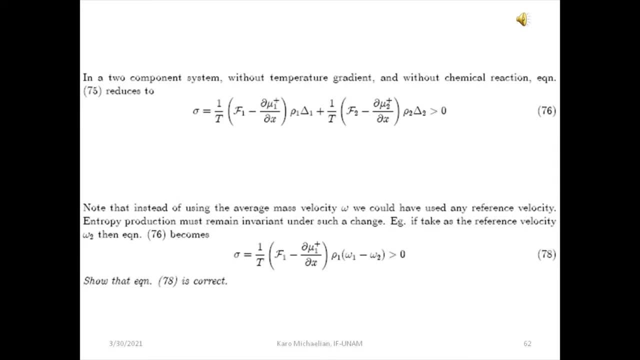 gamma equal to one, gamma equal to two. So we have only the fusion of matter, But we allow forces of the system so we can have electrical potential over the system, for example, And we would have a different force- F1, for component one. 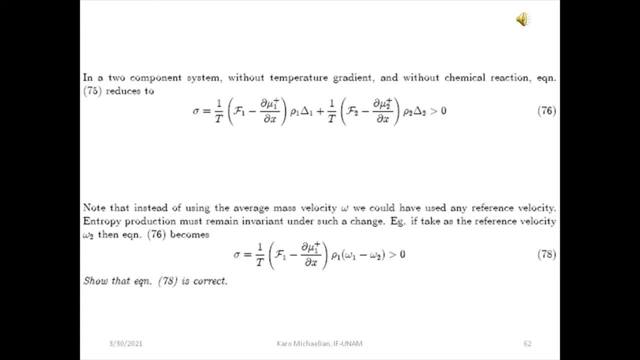 and F2 for component two, because they could have different charge, for example if it was the force due to the electrical potential of the system. But we assume that we have no temperature gradient, so we have no flow of heat in the system. 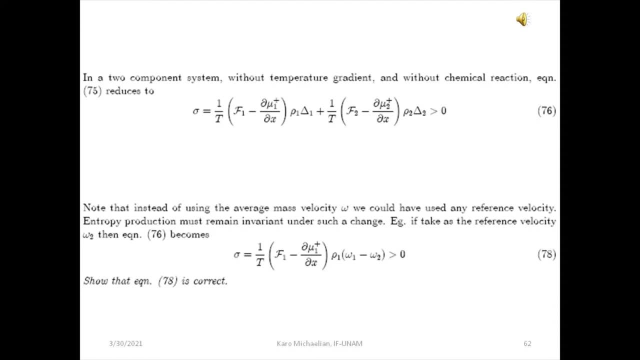 and that we also do not have any chemical reactions occurring within the system. So this is the case of only the fusion of component one with respect to component two for the case of a continuous system, And we'll see that equation 75 reduces to this-